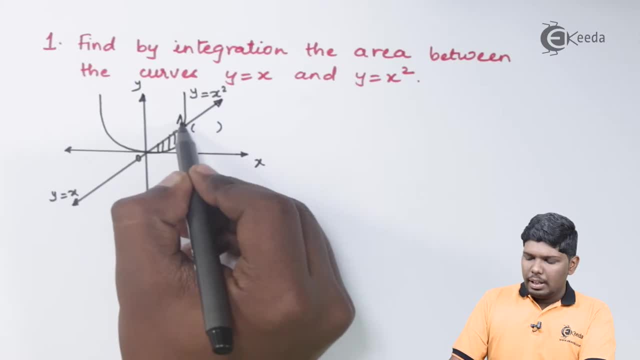 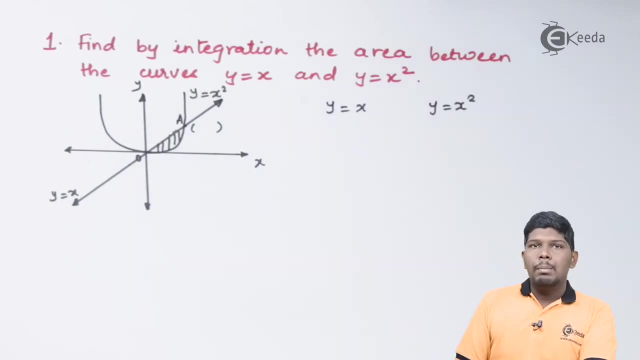 So the first step is to find the coordinates of point A. Considering this as point A, we will first find the coordinates of point A. For that we can simultaneously solve these two curves. Put y is equal to x in this equation. This will give you: x is equal to x square. 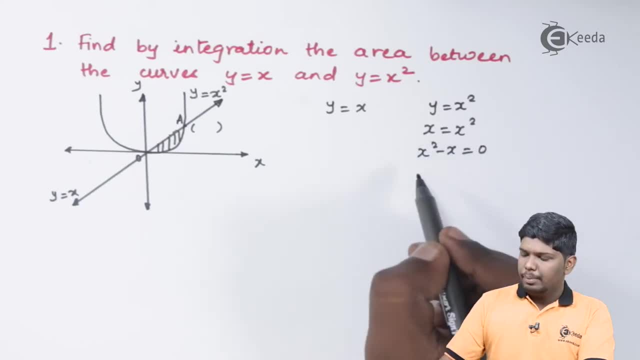 That is x square minus x is equal to 0.. Taking x common, we have: x minus 1 is equal to 0. Therefore, x is equal to 0 and x minus 1 is equal to 0.. On further solving, we have: x is equal to 0 and x is equal to 1.. 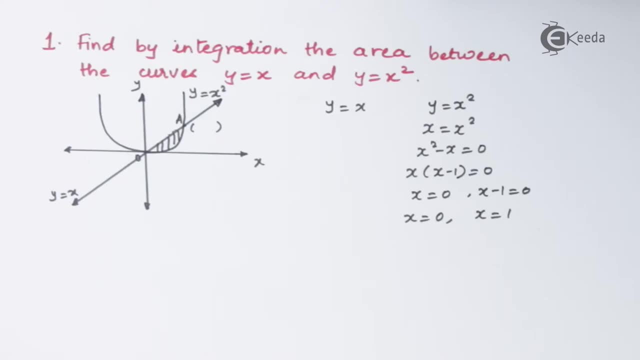 It means the line and the parabola are intersecting in two points, Out of which the value of x is 0 and the value of x is 1.. For that, the corresponding value of y will be obtained from the first equation. Let us substitute: 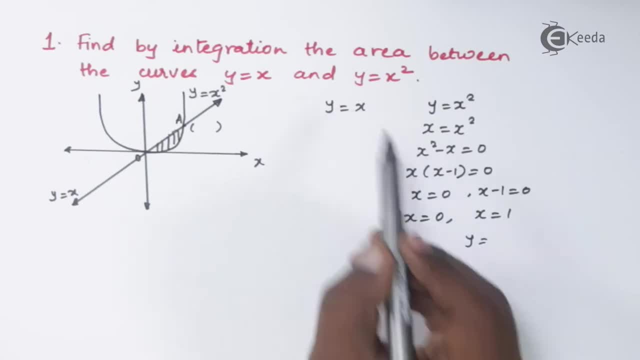 This value of x in this equation. This will give you: x is 0, therefore y will be 0 and x is 1, y will be also 1.. So the first point of intersection is 0 comma 0 and the second point of intersection is 1 comma 1.. 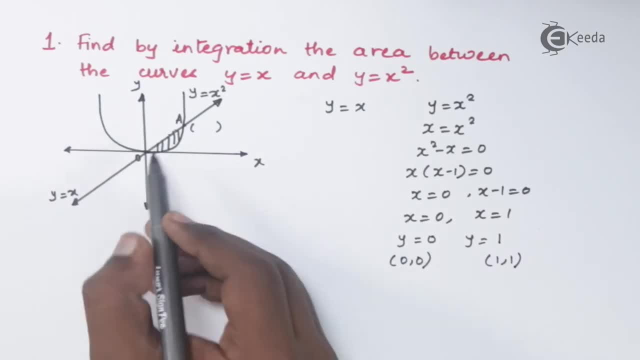 As you can see here also, line and parabola are intersecting. Therefore the coordinates will be 0 comma 0 and the second point of intersection will be 1 comma 1.. So the coordinates of A are 1 comma 1.. 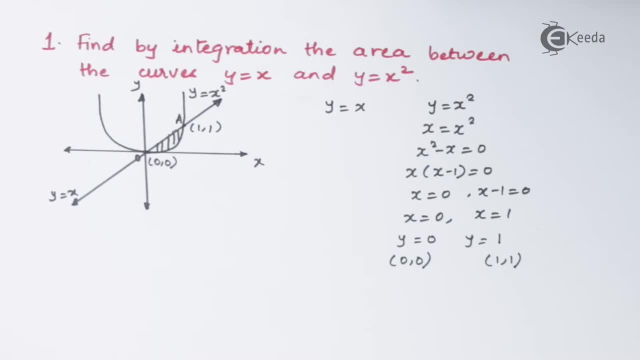 Now, in the next step, to find the area of the shaded region. First, you can consider this line from x is equal to 0 to x is equal to 1.. If I consider the area of the line from 0 to 1. This will give you area under the line formed with respect to x axis. 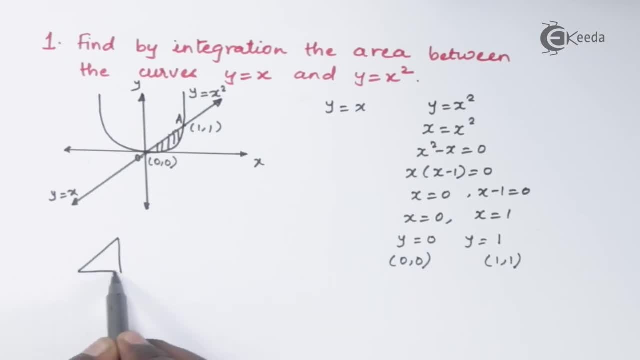 So, in short, this will give you the area of a triangle. This is our line. here the value of x is 0 and here the value of x is 1.. So if I integrate this line, this will give me the area of the triangle. 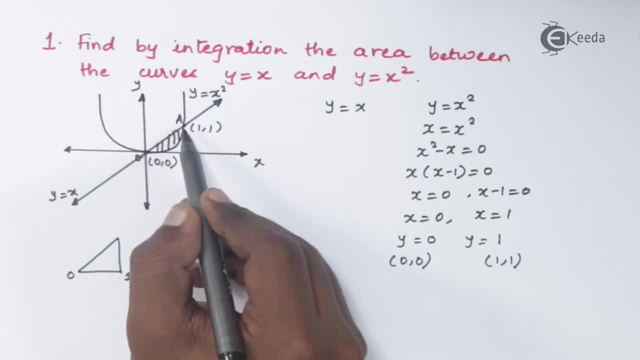 And if I consider the area of parabola again from 0 to 1. This will give you area under parabola. So this will be the region if I calculate area under the parabola again from 0 to 1.. 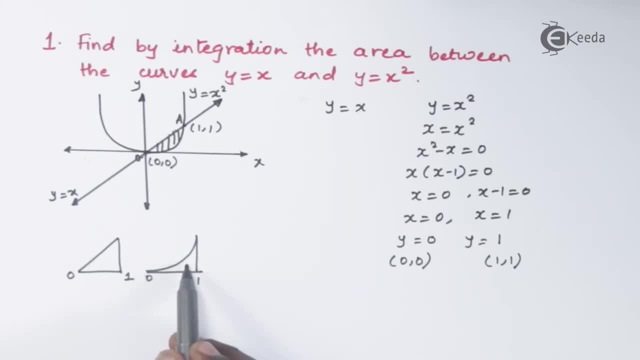 But if you see, I neither require this area nor I need to find this area. I need to find this area. So just imagine that if I subtract these two area, If I overlap this region here, this will become like this: And this part: 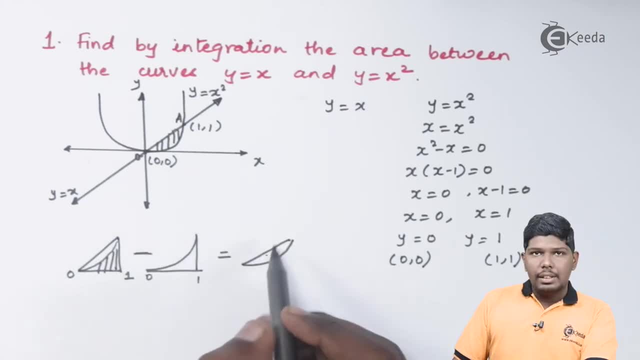 This will be subtracted and the remaining region will look like this, which is the required area. So to find the area of the shaded region, we first need to find area under the line and then subtract it from area under parabola. Both will have limits from 0 to 1.. 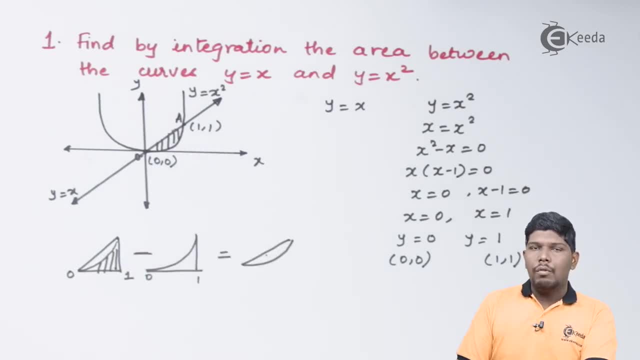 And again we are considering the area with respect to x axis. The formula will be integral: y- dx, The limits of x will be 0 to 1 and the value of y will be obtained from both parabola and line. Here we can write: 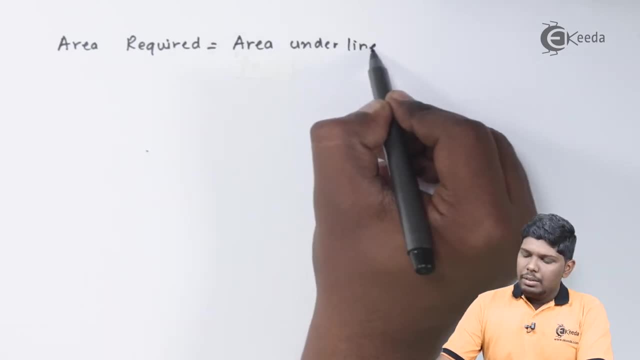 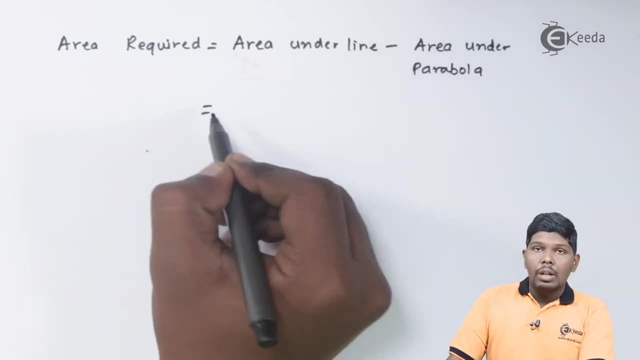 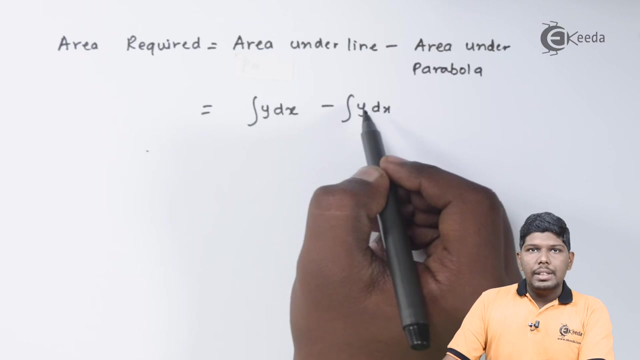 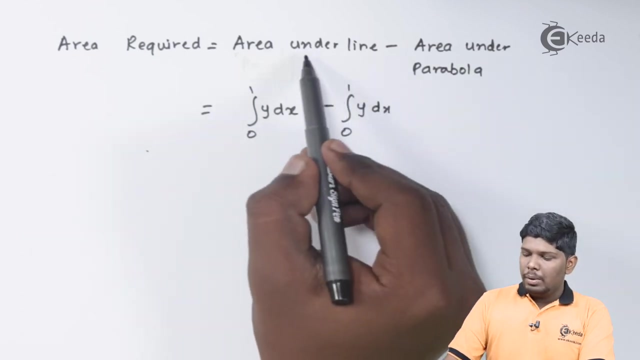 The area required will be equal to area under line minus area under parabola. Both the areas will have formula integral y, dx And both will have same limits, that is, 0 to 1.. But here the value of y will be obtained from the equation of line. 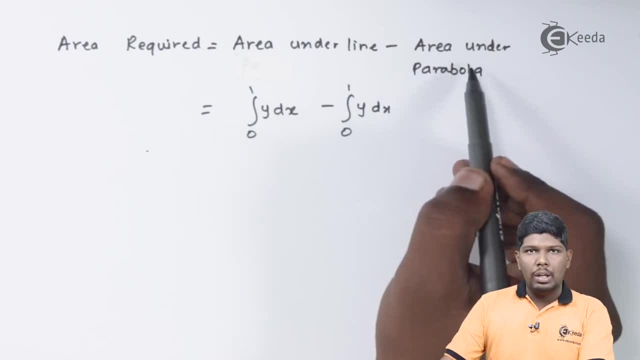 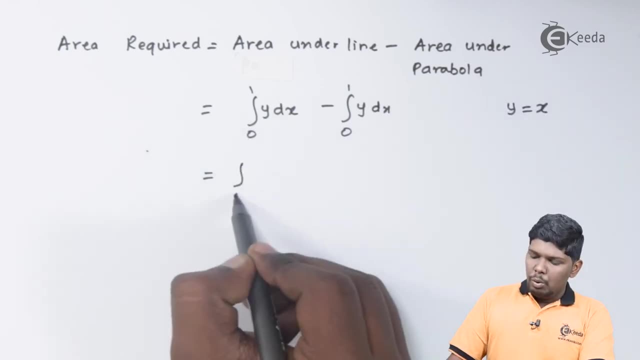 And in the second part, the value of y will be obtained from equation of parabola. As you can see, the equation of line was: y is equal to x. Therefore, this will give you integral 0 to 1.. The value of y is x- dx. 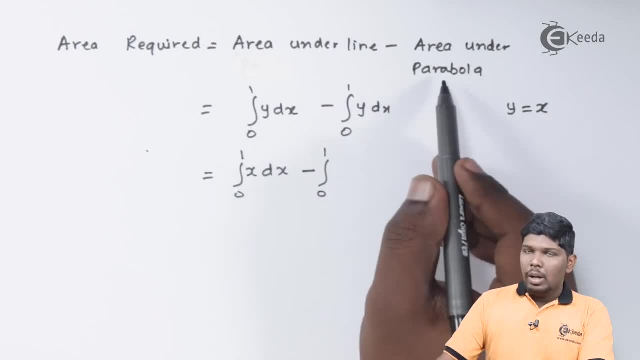 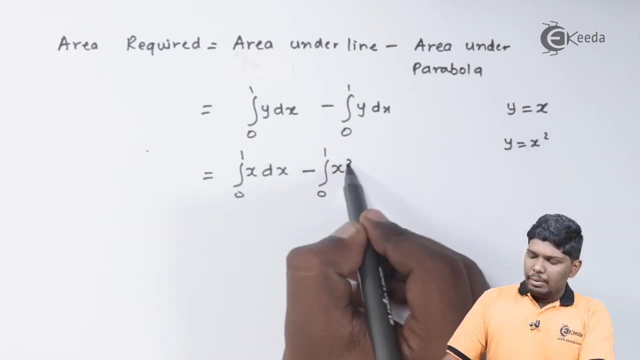 Minus 0 to 1.. In the parabola, the equation was: y is equal to x square, So the value of y will be x square dx. Now let us integrate it. This will give you x square upon 2 minus. 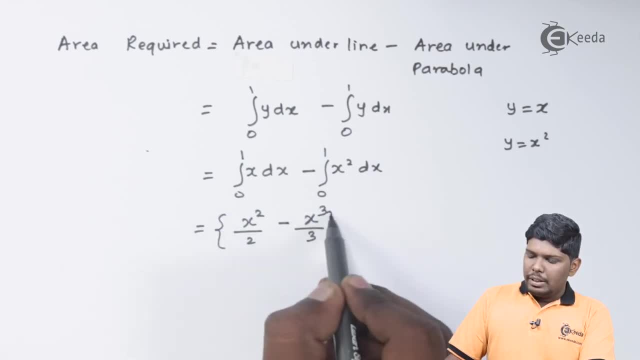 We have x cube upon 3. Both have same limits from 0 to 1.. After substituting the limits, we have 1 by 2 minus 1 by 3.. Minus 0.. 1 by 2 minus 1 by 3 will give you 1 upon 6 square units. 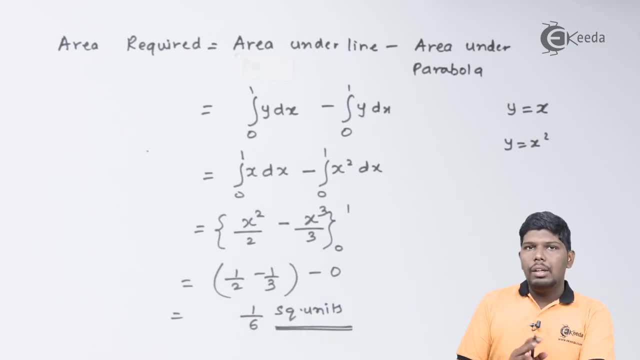 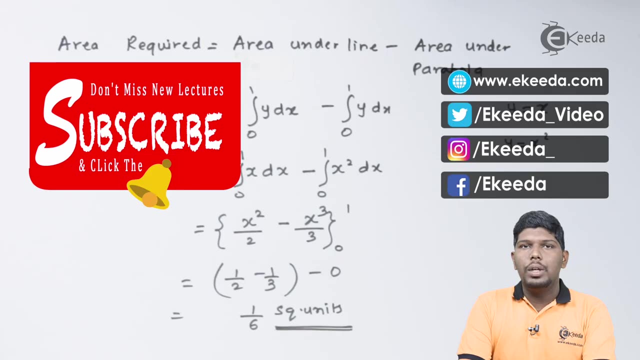 So this is the area which will lie between the parabola and a given line. y is equal to x. I hope, friends, you have understood this problem. Thank you for watching this video. Stay tuned with eKIDA and subscribe to eKIDA. Thank you.